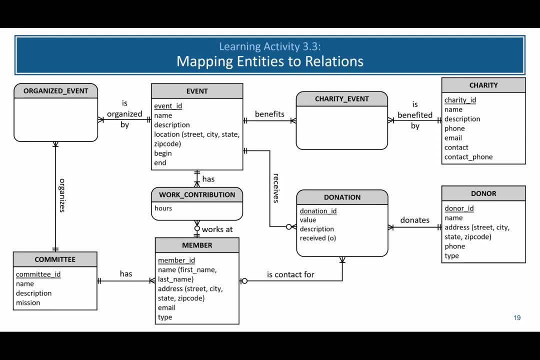 the info icon if you're not sure how to create a relational model, as it will guide you through certain things that you should do. However, the creation is very similar to an entity relationship diagram, with just a few differences, such as domain constraints and the primary key, foreign key pairs. 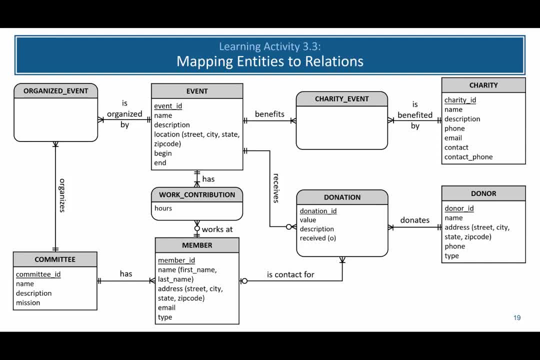 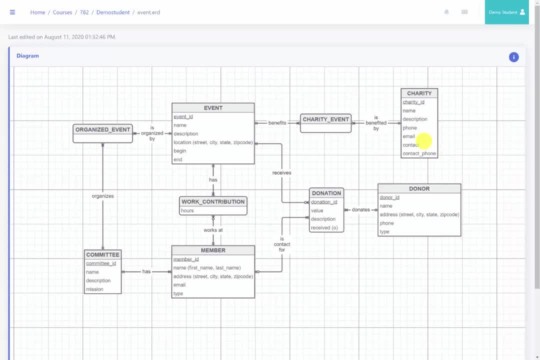 So go ahead and try this on your own, Pause this video and then come back to compare your answers. All right, welcome back. So what I've done here is I've created the slide as an entity relationship diagram on my server. I'm going to go ahead and just copy all this from that page and then we'll. 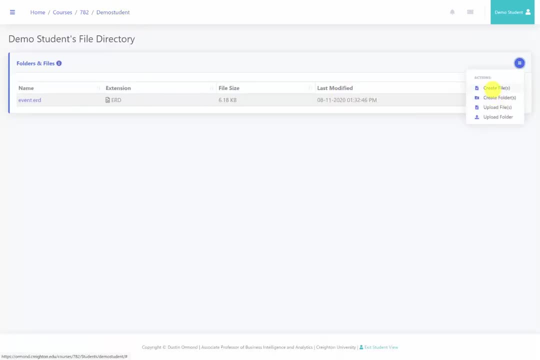 go back to our demo student directory. I'm going to then create a new file and I'm going to call this eventrmrm, and then we'll go back to our demo student directory. I'm going to then create a new file and I'm going to call this event. 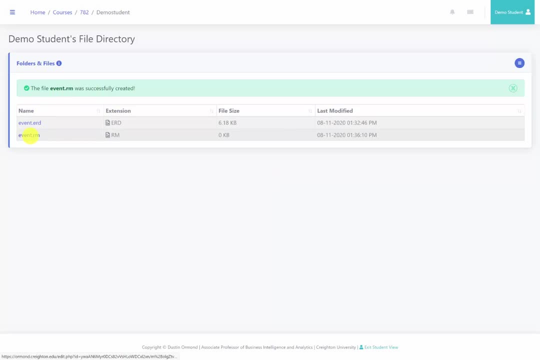 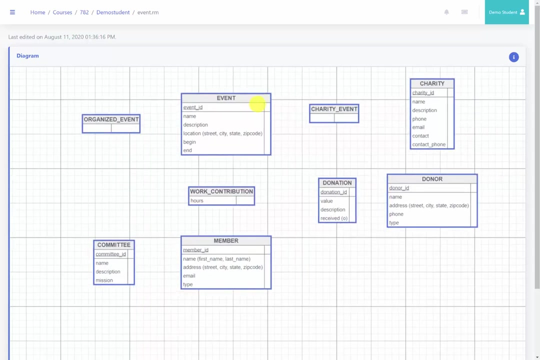 rm. I'll go inside of this file and I will paste the entity relationship diagram. You'll notice that it removed all of the arrows when I pasted it. However, it is now set up for me to easily convert this entity relationship diagram to a relational model. So let's start with. 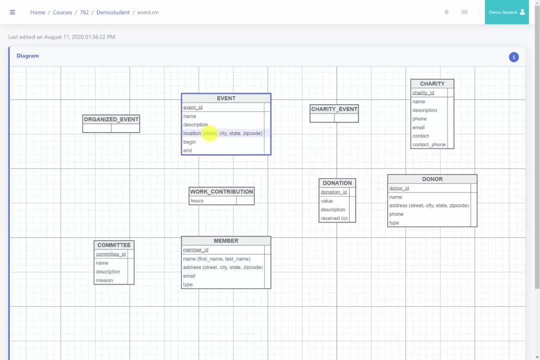 the fields and the domain constraints. So for event, you can see this is a composite attribute that I need to break into its individual, separate components. So I'm going to use this keyboard shortcut of ctrl d to duplicate the field. So I'm going to duplicate it three times. 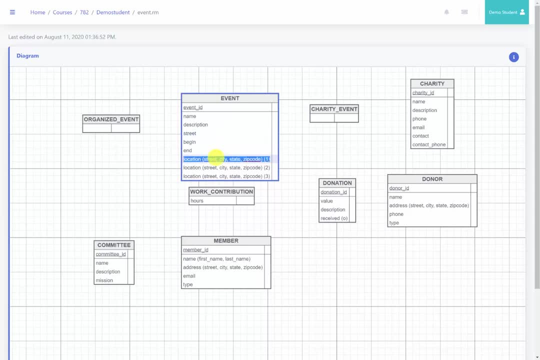 This first one is going to be street, the second one is going to be city and this third one is going to be state and the fourth one is going to be zip code. I'm just going to hold down shift to move city to right after street, just because I prefer it that way. And same with state after city. 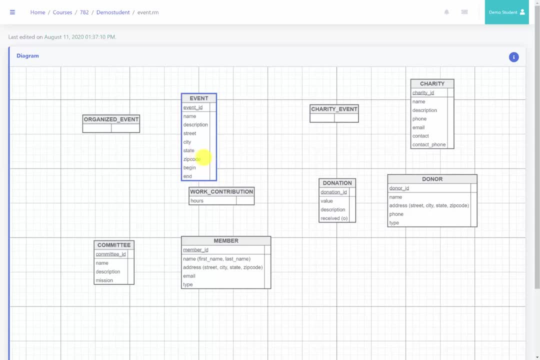 and zip code after begin. Again, the order of these is irrelevant, This is just a matter of preference. All right, so now I'm going to go ahead and add each one of the domain constraints. So for event id, I'm going to use integer. For name, I'm going to do varchar. 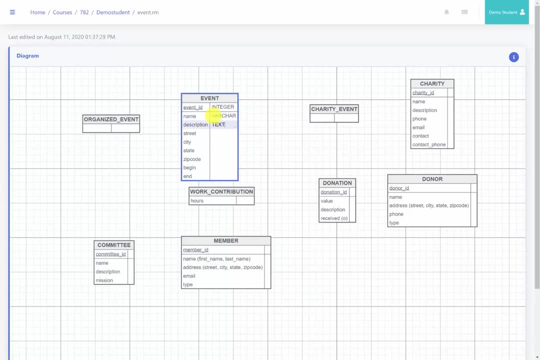 For description. it's longer than 255 possibly, so I'll use the text domain constraint For street. we'll use varchar For city. we'll use varchar For state. we'll use char For zip code. we'll use either integer or char, You decide For begin. this could be. 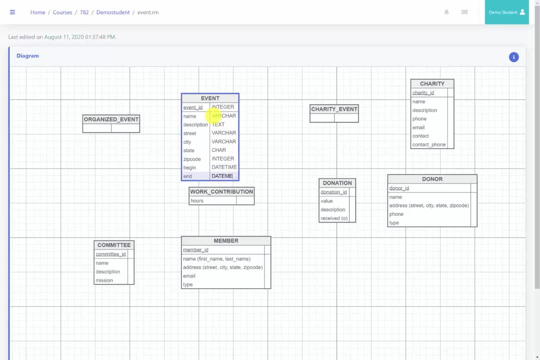 date or datetime. Let's just go ahead and use datetime saying for end Just as a reminder to cycle through these fields. I'm using tab and shift tab All right for charity. since we have only simple attributes here, we don't need to break apart the composite attributes. So I'm 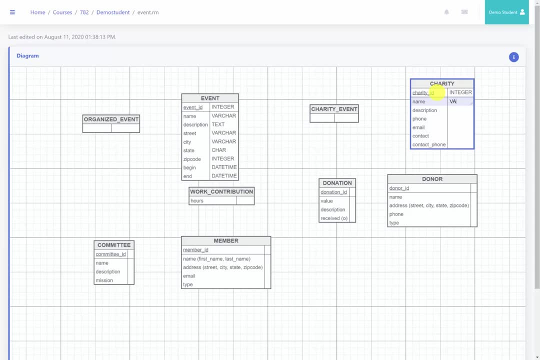 going to use integer for charity id For name. I'm going to use varchar For description. i'm going to use varchar For phone. I'm going to use what is called bigint. Now, bigint allows enough characters for a phone, because integer is not bigint. 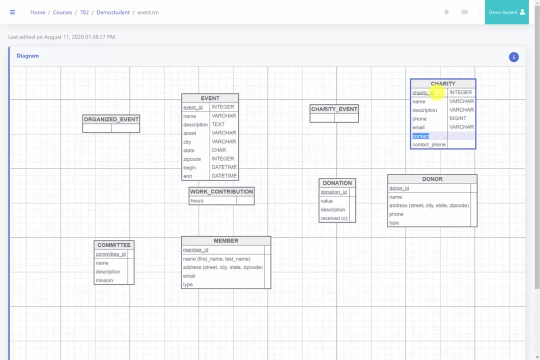 to hold a lot of phone numbers. for email, I'm going to use varchar. for contact, I'm going to use a varchar, so contact is the name of the contact, and then for contact phone I'll use bigint as well. for donor. we have the same issue with 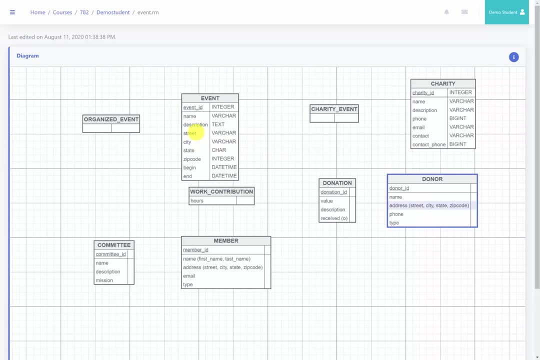 street, city, state and zip code. so rather than duplicating work, I'm going to just hold down control on the street and drag it over here and it should copy that. I'll do the same thing for city and the same thing for zip code, and the same. 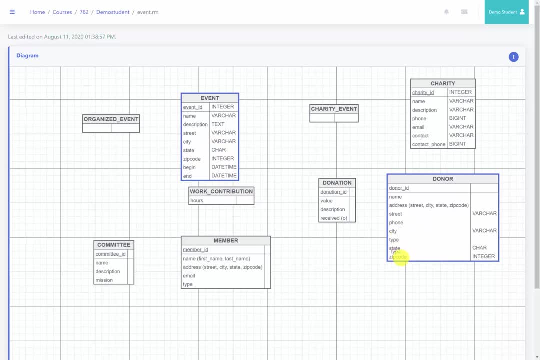 thing for state. I'll go ahead and move type after zip code and I'll move phone after zip code. so we'll go ahead and get rid of address. alright, so for donor ID, we have integer. for name, we have varchar for phone. let's do bigint again for. 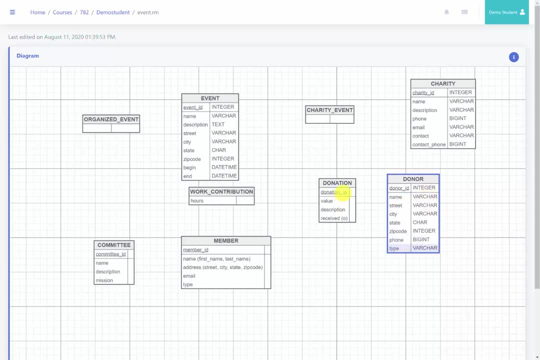 type. we have varchar for donation. we have simple attributes again. so for donation ID, we'll do integer for value. let's do double for description, let's do text for received. let's get rid of that optional flag. we'll use char like 1 or 0, or we could use integer 1 or 0 for. 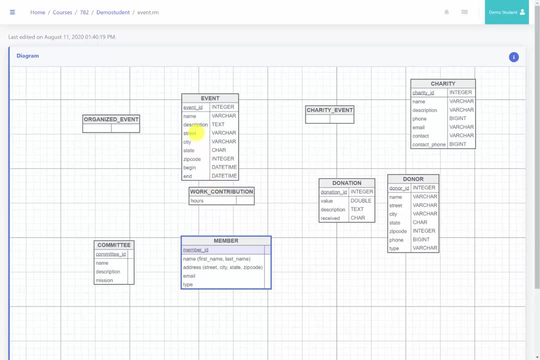 member. I'm going to do the same thing with street, city, state and zip code. so I'll just hold down control and drag Street and I'll drag city and state and zip code. now we'll go ahead and delete the address field and then we'll duplicate the name, drag it up and this first one is going to be first name and 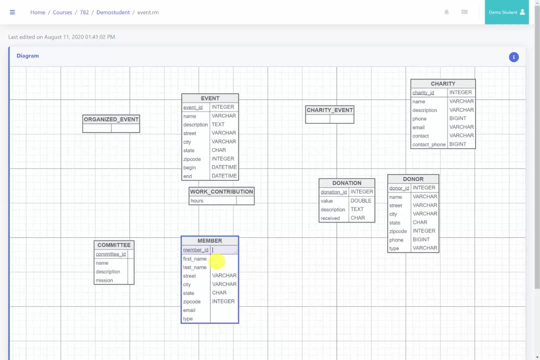 this city and then we'll go ahead and delete the address field and then we'll second one is going to be last name. then for member ID, we have integer for first name. we have varchar for last name. we have varchar. for email, let's have varchar and type: we have varchar. 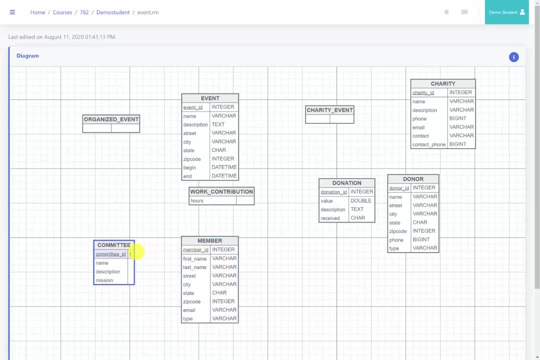 committee is a bunch of simple attributes, so we'll just do integer for committee. ID name is going to be varchar description text mission. let's do text as well for work contribution: the total number of hours someone's contributed. it could be partial hours, so let's do double here. 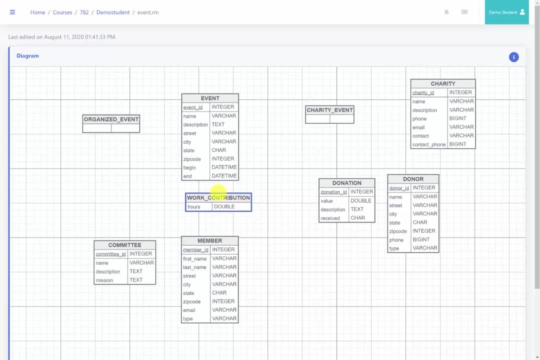 so now what we're going to do is focus on the entity integrity constraints, so each of the ones with underlying values have entity integrity constraints. charity event, organized event and work contribution, however, do not. so charity event should use event ID and charity ID together. so I'm 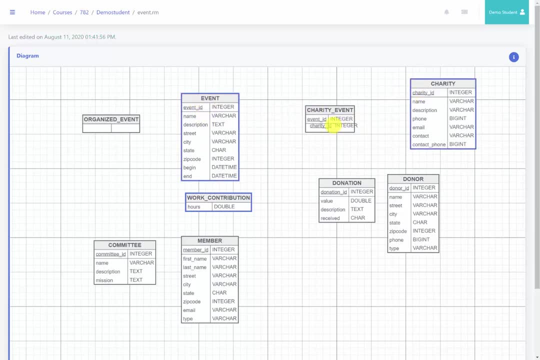 going to just hold down control and drag charity ID and event ID over. we'll just delete this extra field. and then I'm going to take event ID and click and drag it to the ID to create the foreign key, primary key pair- notice how automatically italicized it. and same goes for the charity ID. then for organized event, I'm going to drag event. 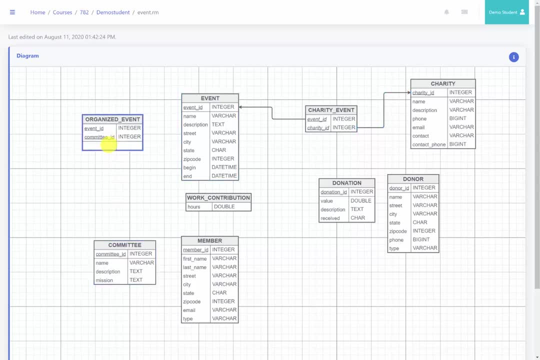 ID over and committee ID over, and together they are the primary key. I will then go ahead and delete that last field drag from event ID to event ID and from committee ID to committee ID to create my primary key: foreign key pairs for work contribution, that is, the associative entity between event and member. so I'm going to hold down control drag- event ID. 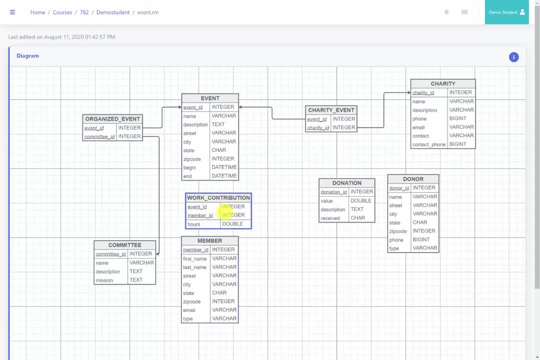 down here and drag member ID up, and that together is my primary key. I'll drag event ID to event ID and I'll drag member ID to member ID for my primary key- foreign key pairs. between committee and member. we have a one-to-many relationship, so I'm going to take the committee ID and I'm 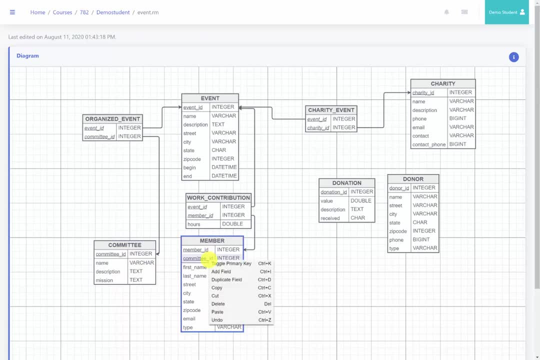 going to drag it over to the member. it automatically made it part of the primary key because it was a key on the other side. I'll just toggle this as a primary key. I like my foreign keys at the bottom. this is a matter of preference. it's not necessary for you to do that then. what I'm going to do is: 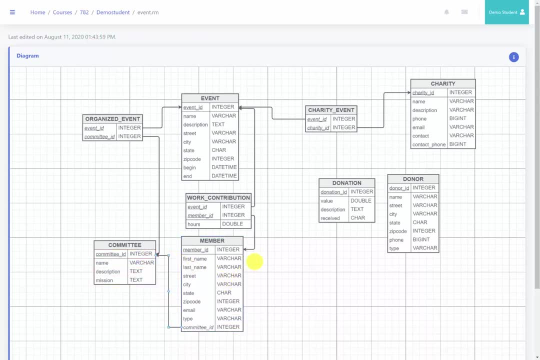 drag from committee ID to committee ID indicating the primary key for key pairs for donation. what's involved is a donor, a member, an event. so I'm going to take the primary key of member and I'll move member ID over, I'll move event ID over and I'll move donor ID over. now the three of these: